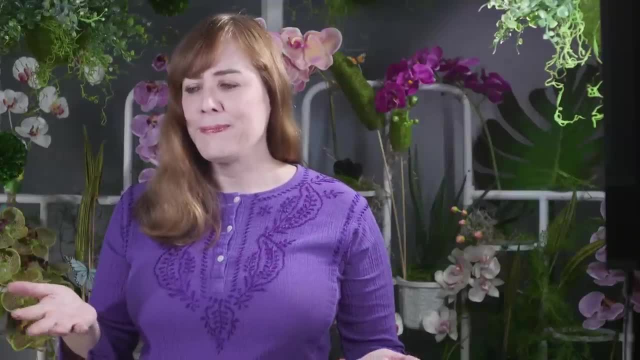 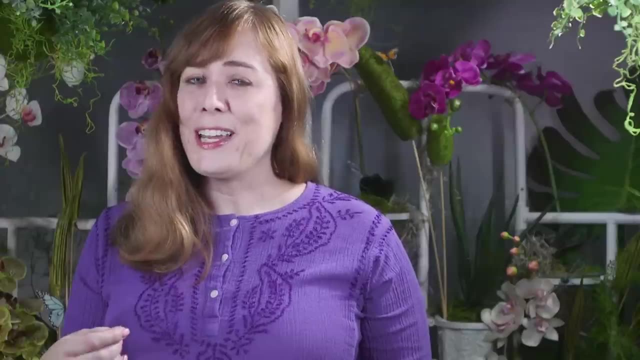 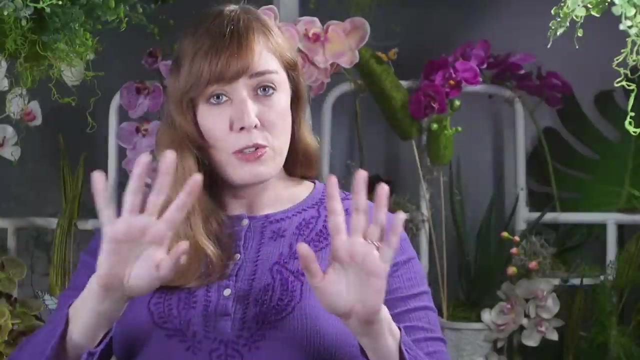 and they perform the actions you associate with a dog Wagging a tail, running around on four paws, biting and barking and panting. Similarly, in biological molecules, the carbon skeleton determines their general 3D shape, but what's on the surface of the molecules determines their 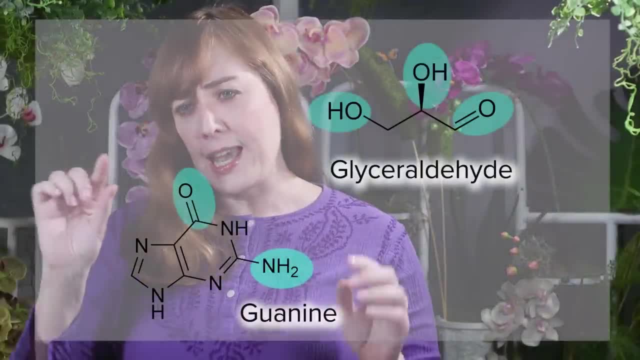 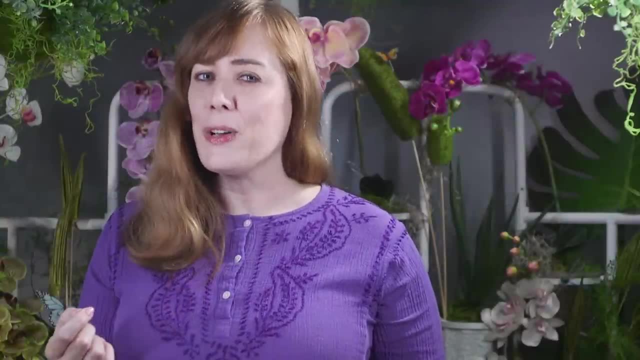 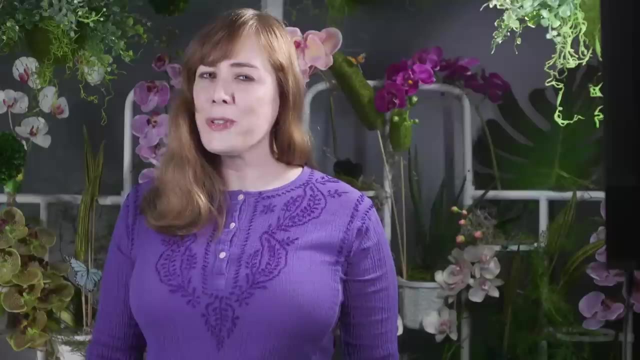 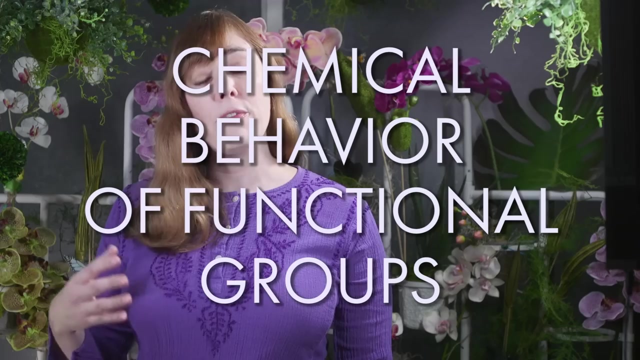 chemical behavior. Small chemical species hanging off from the exterior of these molecules bump into each other and react. These are known as functional groups. To understand what kinds of chemical reactions biological molecules can do, you have to understand the chemical behavior of the functional groups on the surface of the molecule. 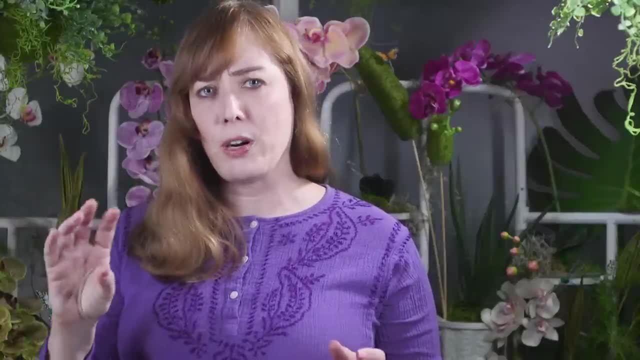 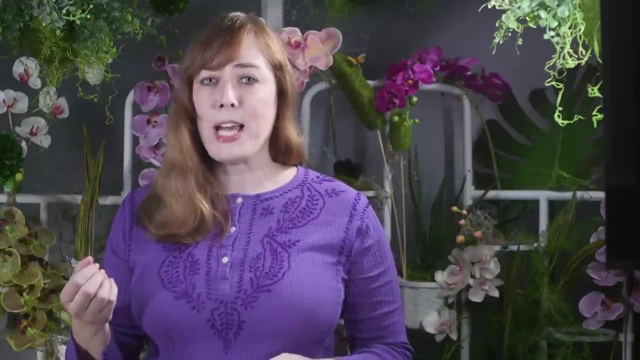 For instance, if a molecule has a big patch of functional groups that are hydrophobic, that side of the molecule is going to repel water. It's going to behave very differently from a patch of acidic functional groups or basic functional groups or functional groups that 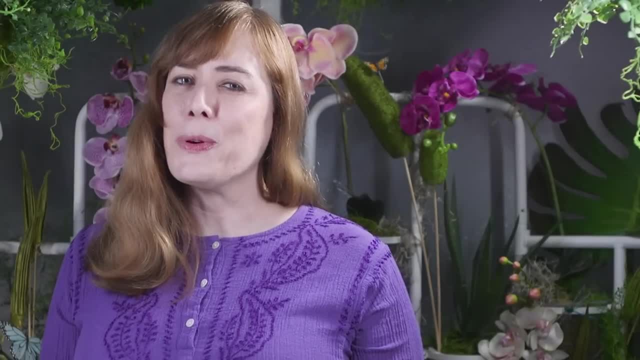 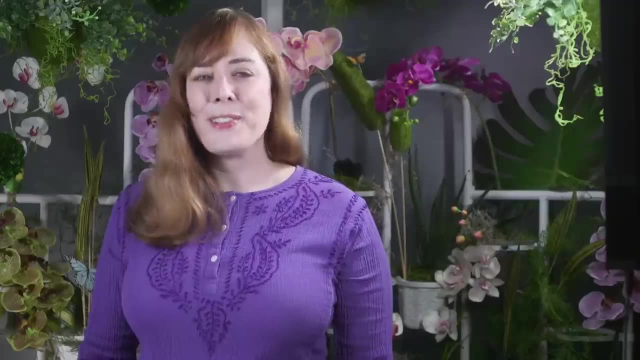 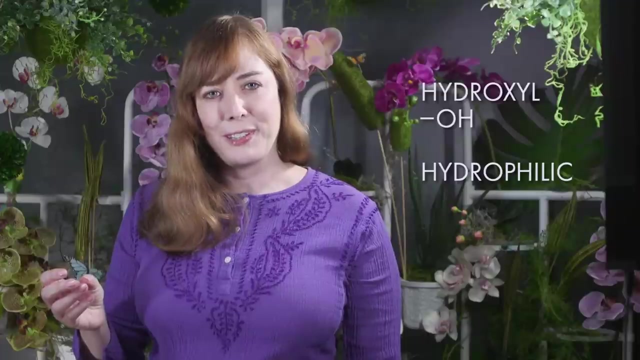 bond to each other for a long time bridges. Let's look at the most common functional groups. OH is the hydroxyl group. This group is hydrophilic, so if a molecule has a patch of OH groups, that region will be hydrophilic. These are highly reactive groups participating in 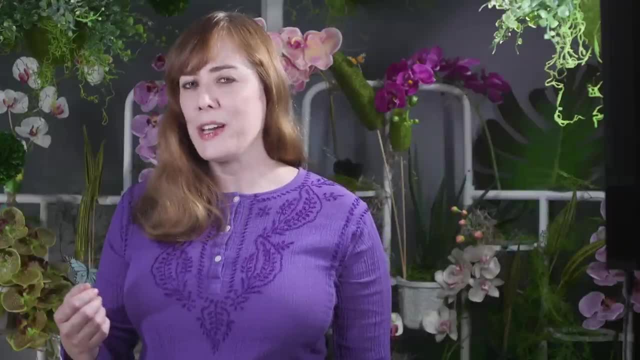 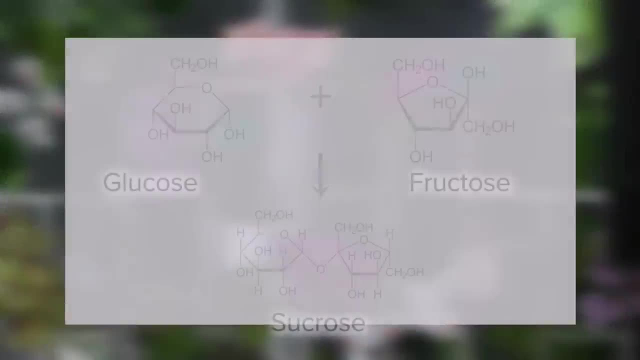 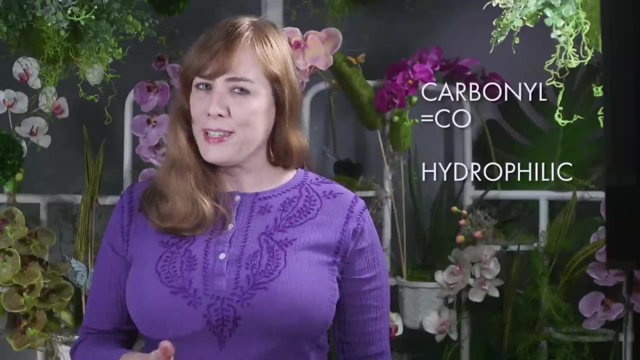 a variety of chemical reactions. One place you'll see the hydroxyl group is in dehydration reactions that link polymers together. Here you can see how hydroxyl groups are involved in these two sugars joining together. The carbonyl group, CO. this is a carbon double bonded to an oxygen. This is a polar group. 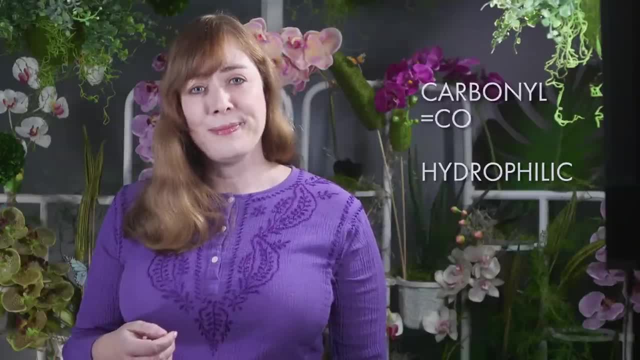 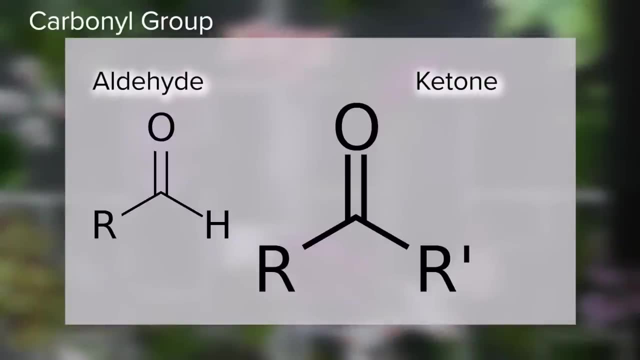 that will increase solubility in water. If this group is at the end of a carbon skeleton, it's called an aldehyde. Otherwise it's called a ketone. These are groups that you're going to see in sugars, For example. here's a. 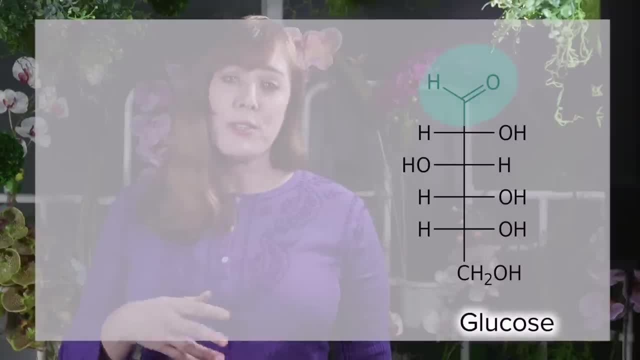 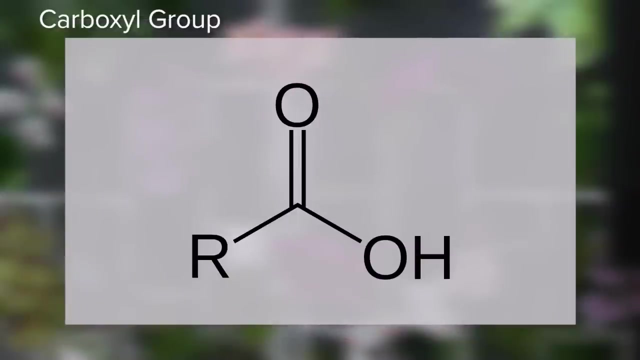 carbonyl group that we'd call an aldehyde at the end of this glucose molecule. And here's a ketone group on fructose. You can see how it's not. on the end, Carboxyl group is COOH, so you have a carbon double bonded to an oxygen. 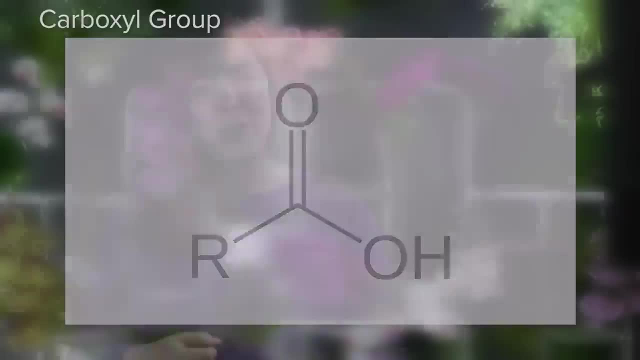 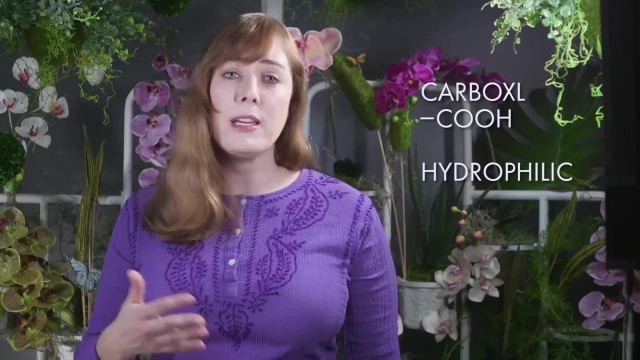 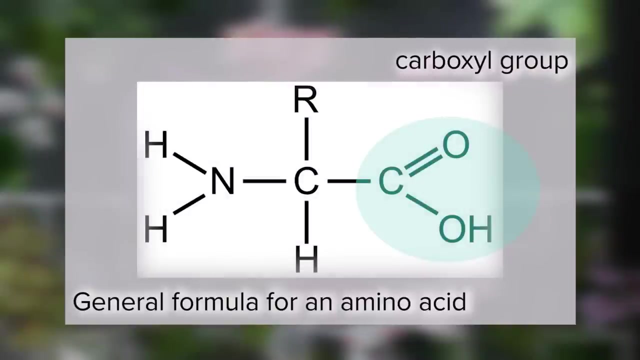 and also attached to a hydroxyl group. These groups confer acidic behavior to molecules because they tend to donate their H+, becoming COO- You'll see these on one side of amino acids, for instance, And on the other side of an amino acid you see the amine group NH2.. 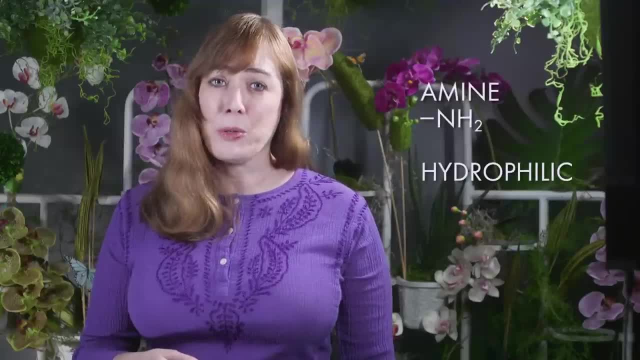 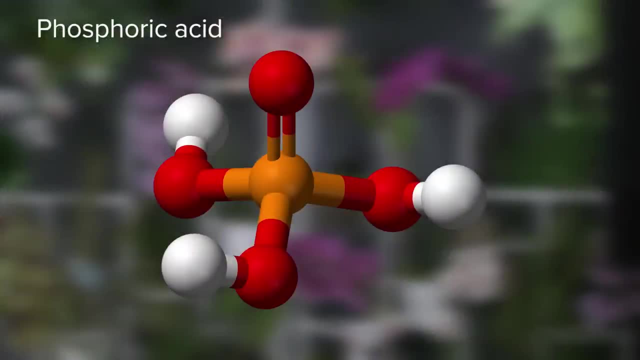 The amine group confers basic behavior to molecules because it tends to accept NH+ becoming NH3+. The phosphate group loses H+ ions to become PO4 3-. So again by increasing H+ concentration, it's acting as an acid. 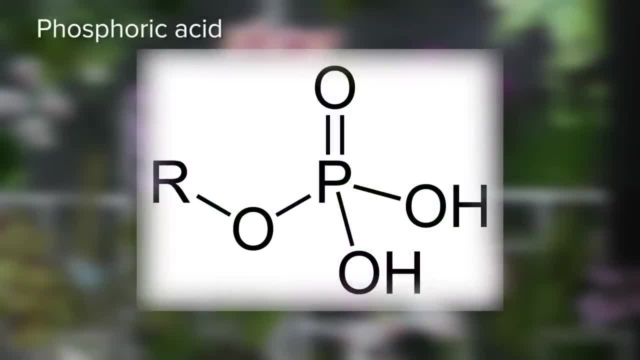 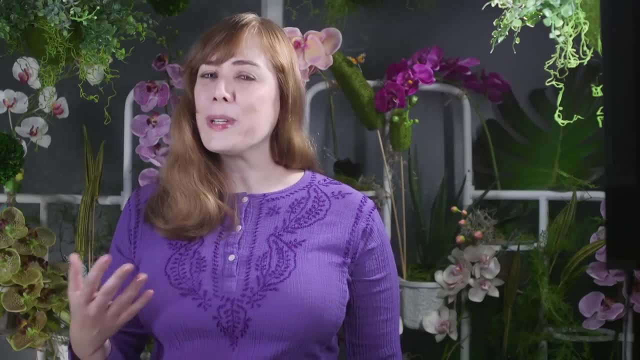 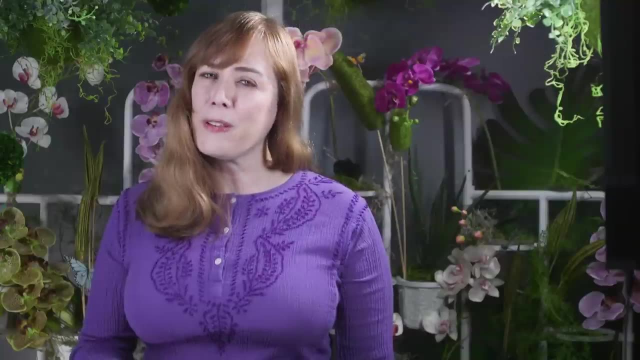 This functional group is attached to the carbon skeleton by its oxygen. Then you get a phosphorus and then three other oxygens. Phosphates are also really important in energetic reactions, For instance those involving the molecule ATP, For a lot of reactions. 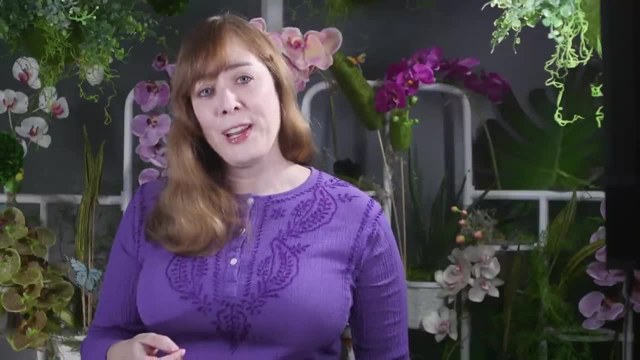 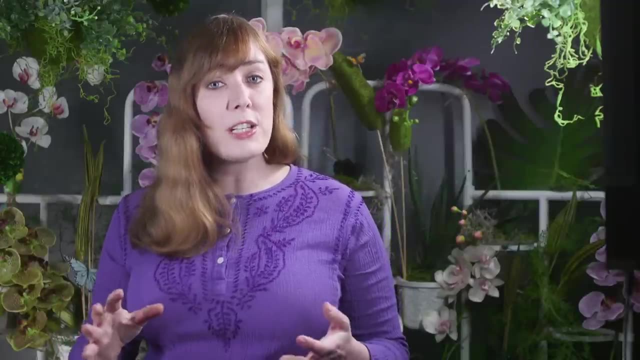 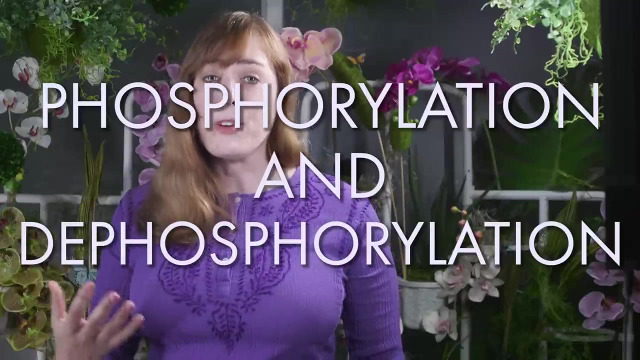 the controlled adenine. the controlled adenine- the controlled adenine additional- of a phosphate group is used to either store or release energy, or sometimes the addition or removal of a phosphate group changes the conformation of a molecule. So you'll hear about phosphorylation or diphosphorylation. 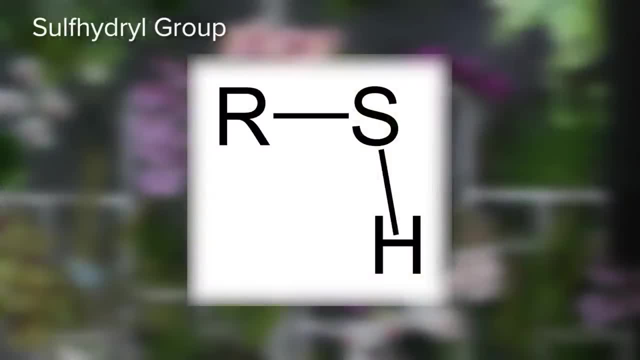 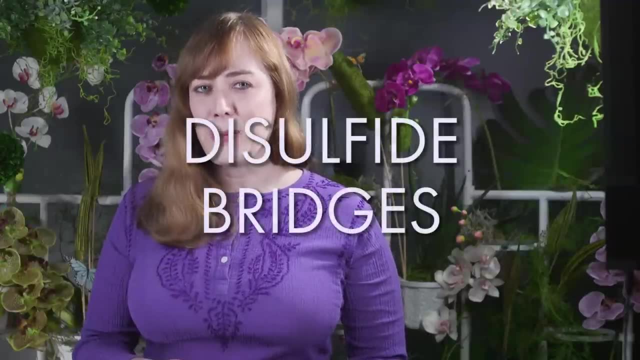 The sulfhydryl group is SH, a sulfur atom bonded to a hydrogen. Sulfhydryl groups tend to bond to other sulfhydryl groups, forming disulfide sulfide bridges. This is important in protein folding joining together two. 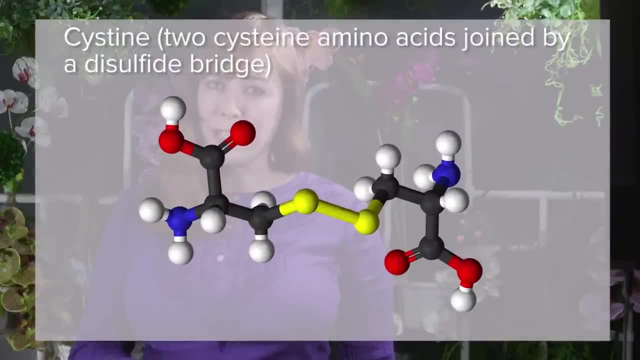 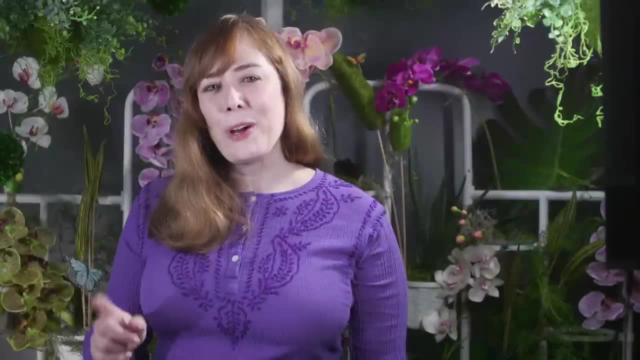 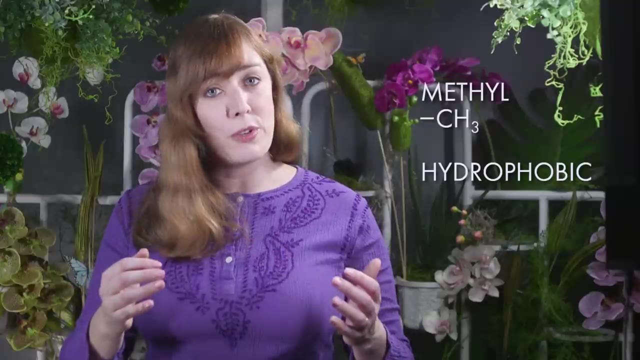 regions of an amino acid chain in a stable conformation. The methyl group CH3,. this is the one functional group we're going to see today that is hydrophobic. So if you see a patch of methyl groups on the surface of a biological molecule, 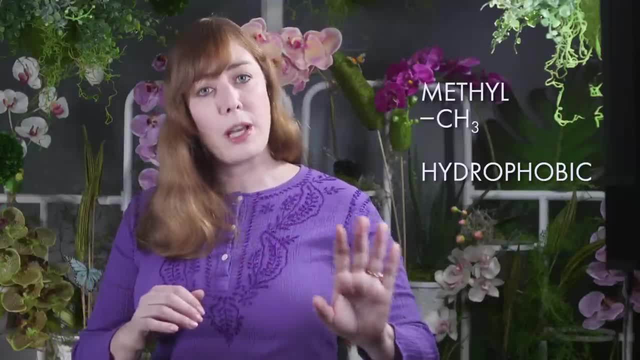 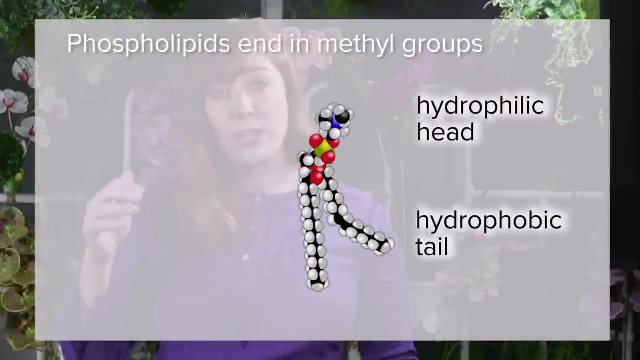 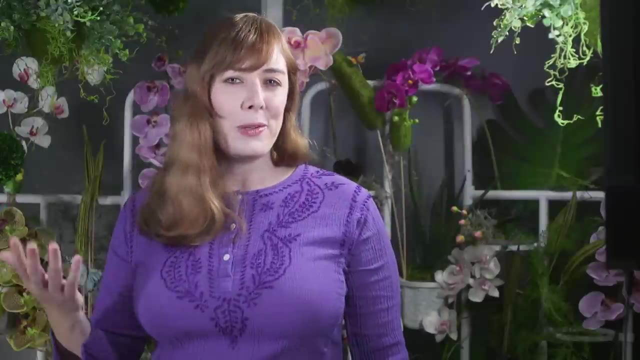 that region is hydrophobic and will repel water. Think of molecules like phospholipids. This top part, with a phosphate group, is hydrophilic, but these tails, which are hydrophobic, end in methyl groups, Compared with these other.